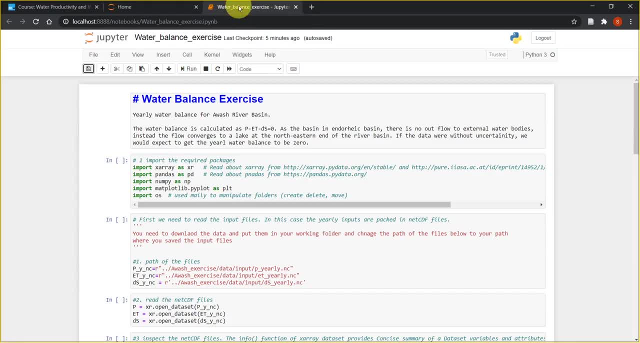 And start Jupyter network and open the water balance exercise Jupyter notebook file which I have it on In the data. there are two folders: input and output folders. The input folder where it contains all the input required to calculate the water balance, and the output folder is to save some of the output results later on. 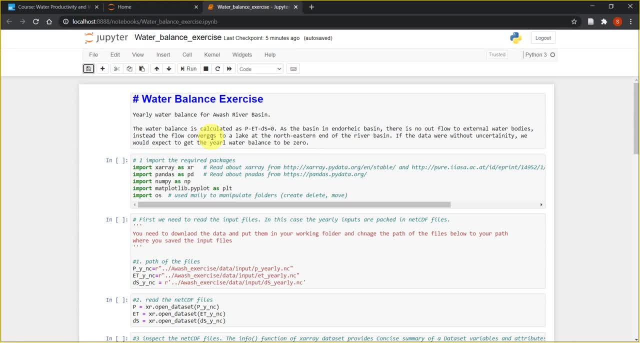 So we are going to calculate the yearly water balance for Awash River Basin. Awash River Basin is a basin which is located in the eastern part of Ethiopia. Awash River Basin is an indoor HEC basin or a closed basin, Meaning there is no known. 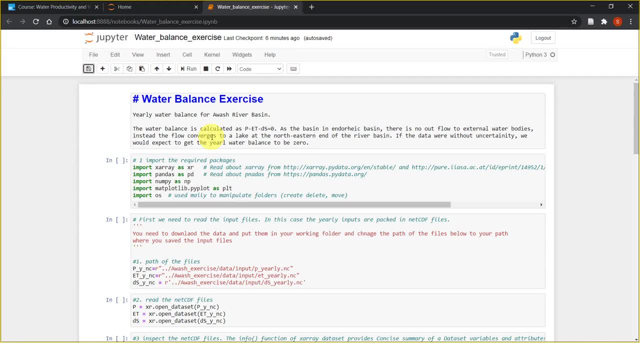 outflow to external water bodies from this river basin river basin. Instead, all the flows converge into a terminal lake at the northeastern end of the river basin. So for such kind of river basin, the water balance is simply calculated using the input, which is a precipitation. 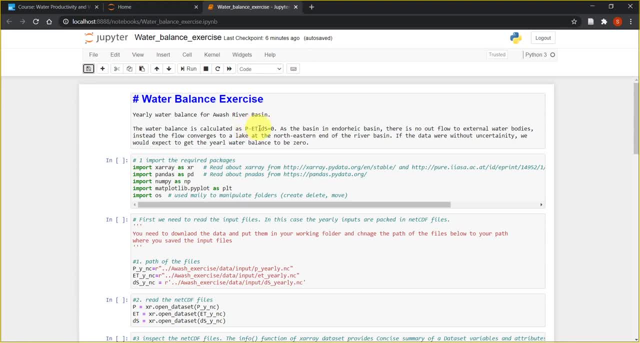 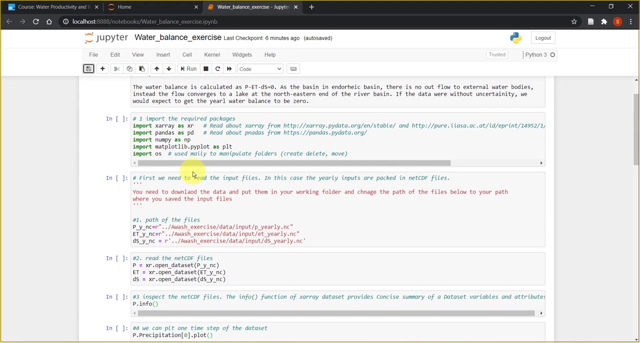 minus the output in the form of evapotranspiration, which should be equal to change in storage, or simply precipitation minus evapotranspiration minus change in storage, is equal to zero. For the exercise, I downloaded the precipitation and evapotranspiration data from VAPOR database and calculated the yearly precipitation and 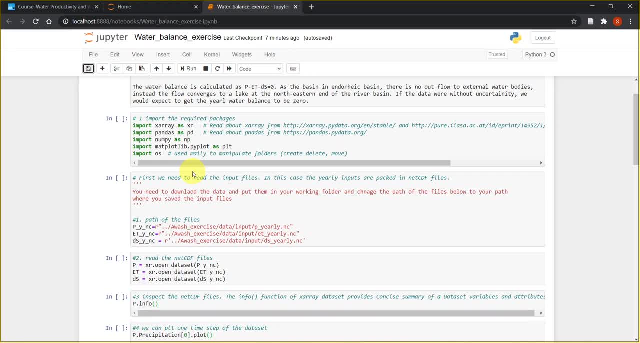 evapotranspiration for the yearly 2009 to 2015 and also download and calculate the change in storage from GRACE products for our Schreber basin. So first we need to input the required package, which are shown here, If you are. 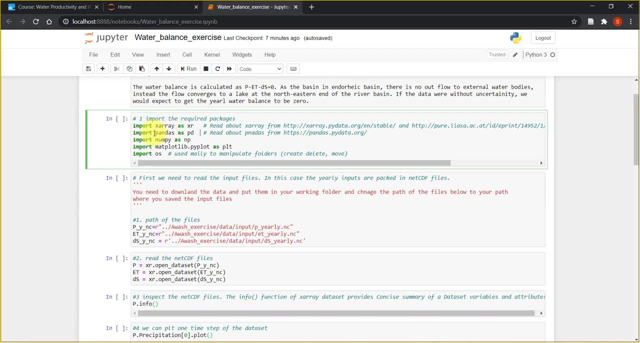 not familiar with X-array or Pandas library, which are very important ateur analysis of spatio tempura data. I recommend you to go and read and get familiarized with this package. I have put some of the links here or you can google them in you rate and understand the use of these packages. So first we 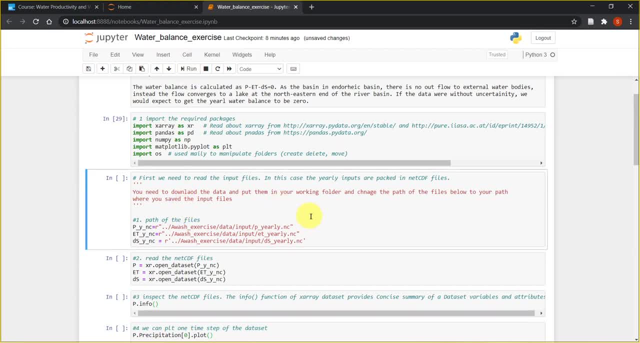 to import the required packets and the next is to get the paths of the input files. so the input files are these three netcdf files which contain the yearly spatial data for precipitation, evap, transpiration and change storage. i have put them in a folder power exercise and then the data folder. 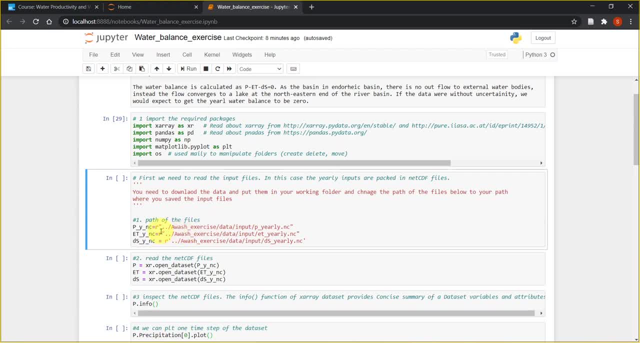 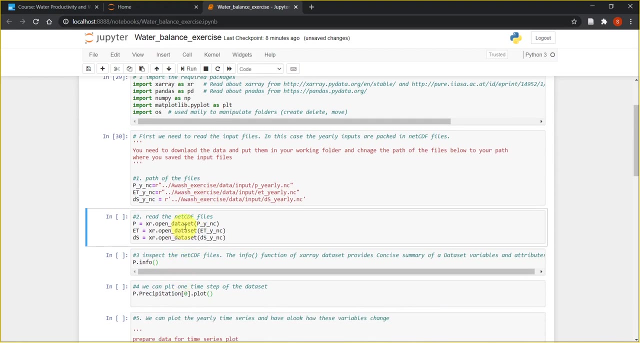 but for your case the paths could be different. so please make sure that you have the right paths for the, the three inputs. so let's get run and get the paths to the files and open the files in xrA. so we have now three data sets called p for precipitation, et for evap transpiration and 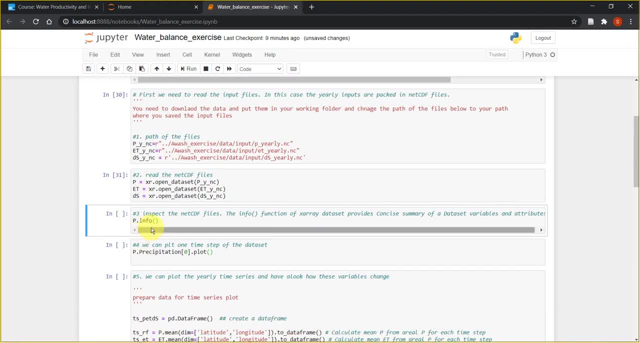 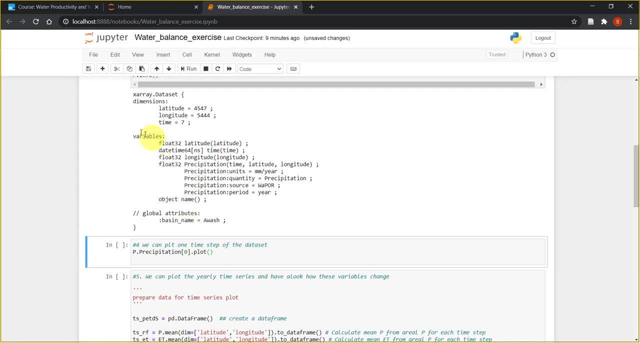 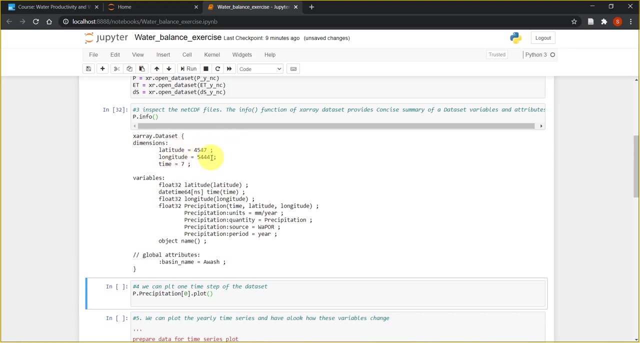 ds for changing the storage in xrA. you can inspect, you can get some summary of the data. so, for example, for precipitation, if i have pinfo, if i run this command, i would get some summary of the data which says: this data is latitude and longitude coordinates of this march and time of magnitude 7, so 47 is starting from 2009 to 2015. the variable is 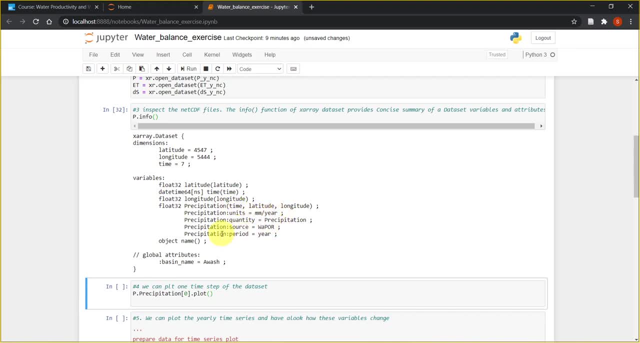 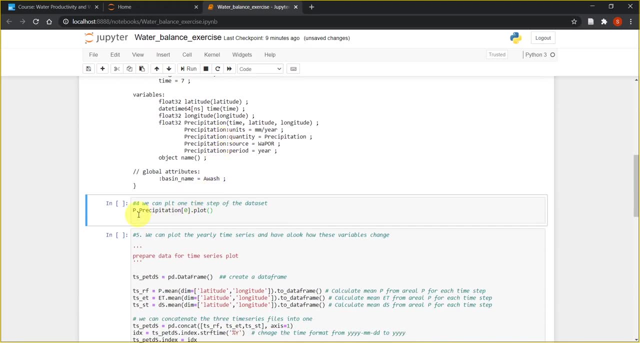 the unit is millimeter per year, source of the data is vapor and the time step is year. that means a yearly time step. we can also upload and observe the spatial variation of this variables. so, for example, if we plot precipitation, p precipitation and the zero is to indicate the. 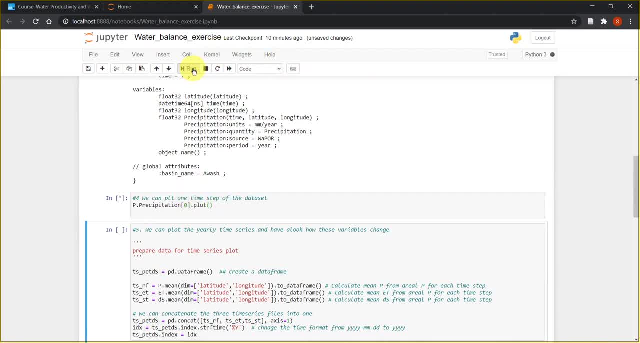 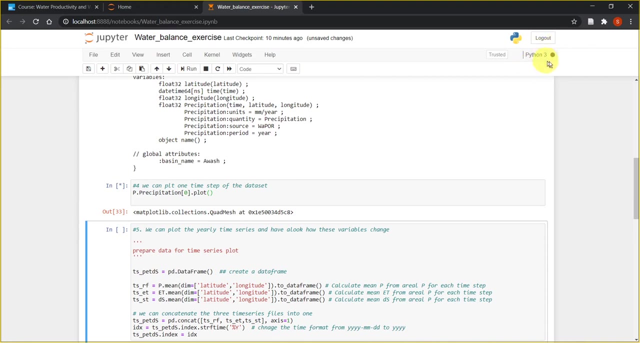 first year plot: precipitation: p precipitation and the zero is to indicate the first year plot. if we run this, python would take a bit time because the file size is relatively big. you can see python is busy here. if you see this black dot, that means the file is busy, so we need to wait a bit. 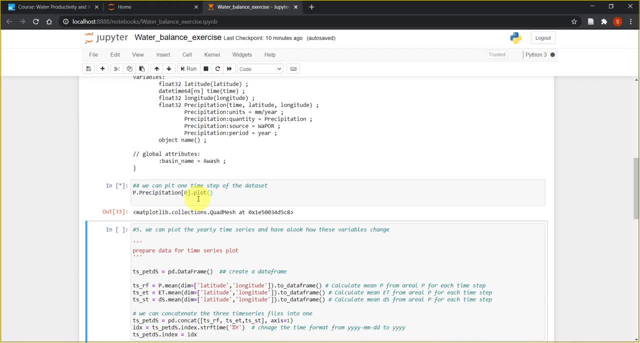 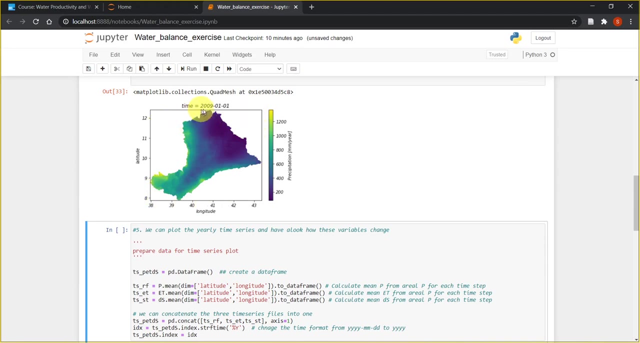 yeah, now we have the plot of the precipitation for the year 2009: latitude, longitude and the magnitude of the precipitation. so, as you can see, the northeastern part of the basin, which is actually the lowland part of the basin, receives less amount of rainfall- less than 400 millimeter per year, whereas the 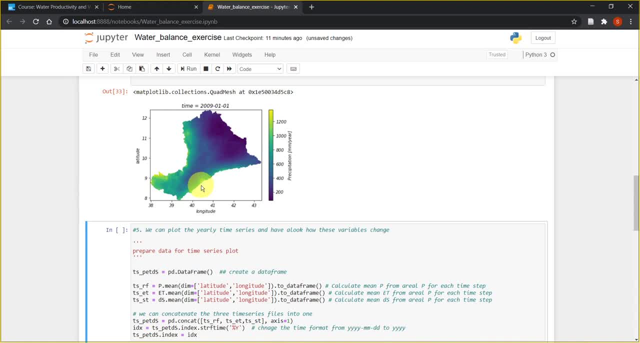 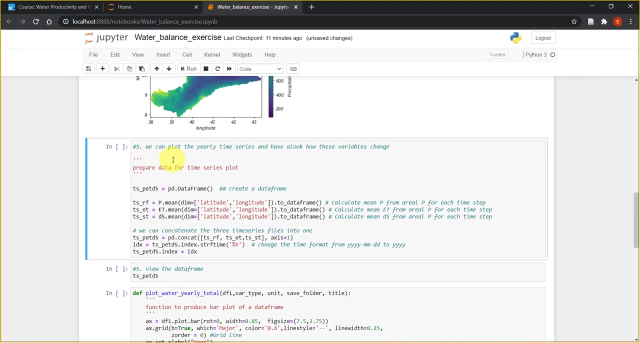 western and southeast part of the river basin receive a relatively high amount of rainfall, more than 1200 millimeter per year. so we can do the same for the other parameters and see how those- evapotranspiration and also changing storage- vary spatially. next we can plot the yearly time series of these variables. so to do that we need to first 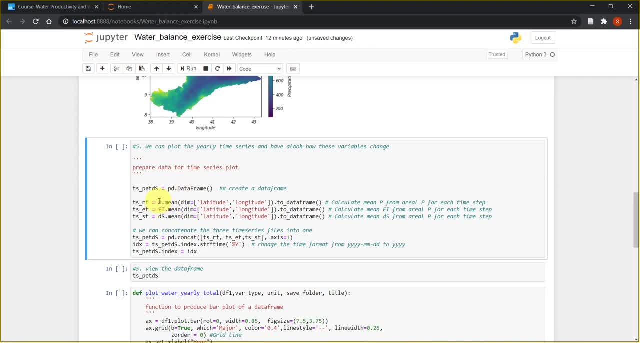 calculate the spatial mean of each variable and save them into a data frame. so we can do that using pandas. so if we say, calculate p dot mean and the dimension, latitude and longitude which calculate the special mean of precipitation for each year and also for evapotranspiration and 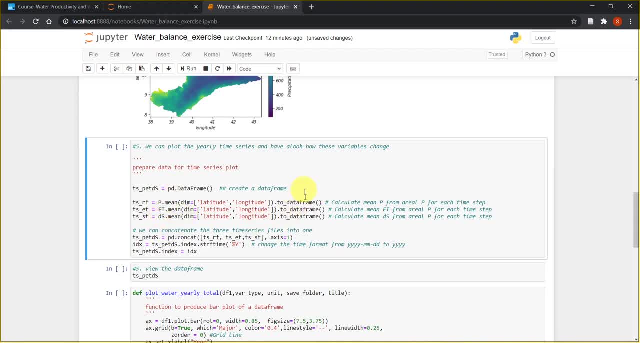 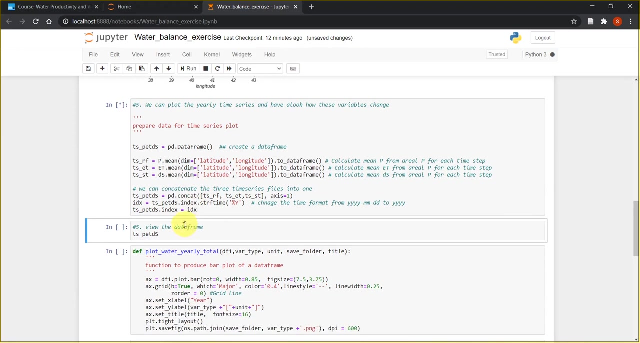 changing storage and save them into a data frame. so if you run this also, it would take a bit of time because it can't should calculate the special mean for each variable for each year. once this is finished, we can view how the data frame looks like. come on, python, be a bit faster. 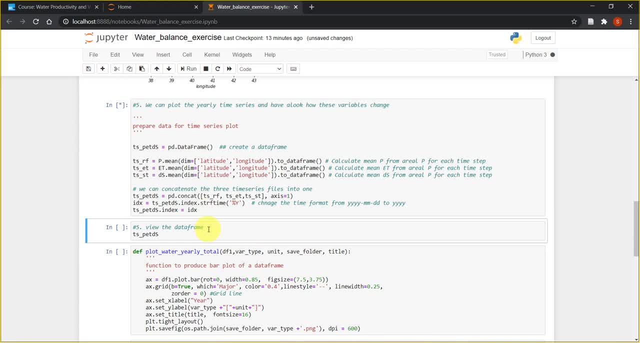 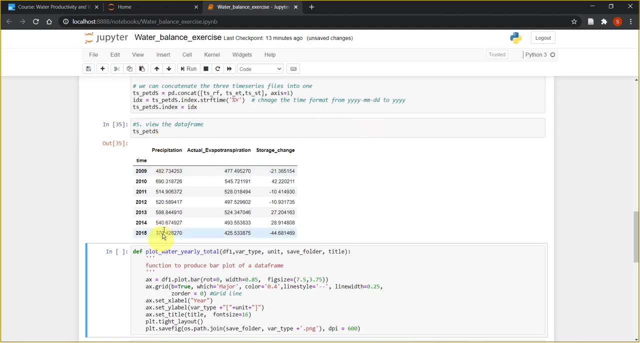 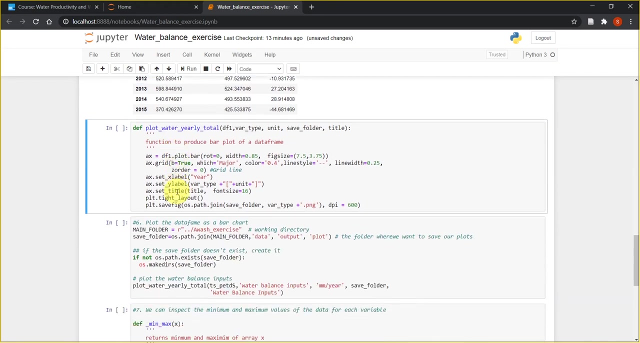 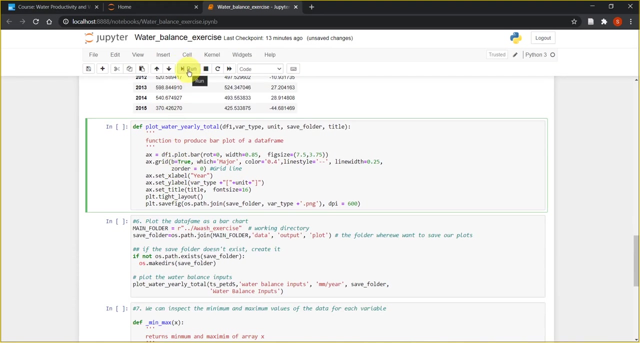 right, let's call it okay. yeah, now it's finished. let's run this path and see. yeah, so you can see this data frame has three columns: first column, precipitation. second column, actual evapotranspiration, and said to call them storage change for each year. so we can plot a bar chart of this data using the plot function. I have this function to plot. 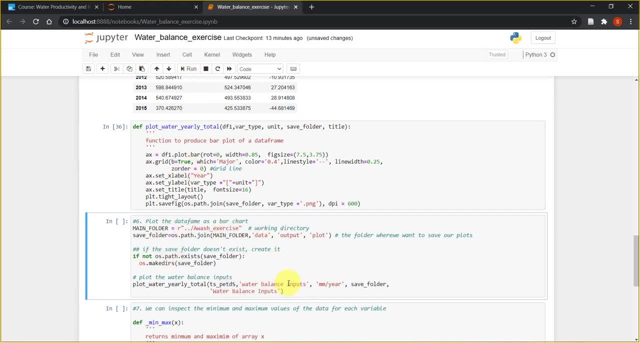 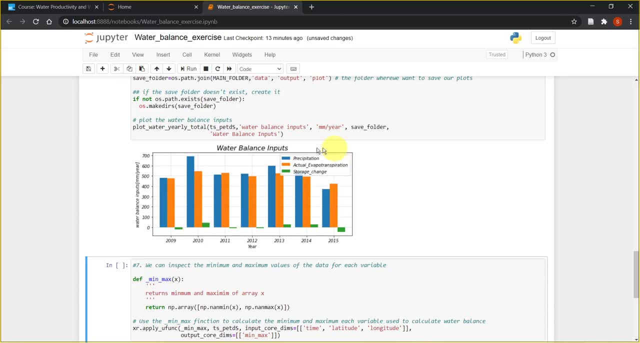 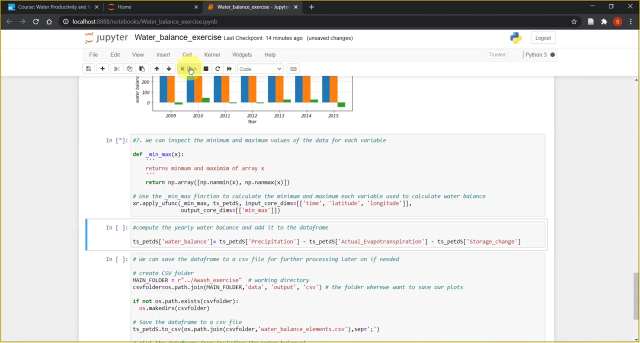 and give the path and some customization of the plot. and so if I run this, I would get this plot which shows in the y-direction the magnitude of each water balance inputs, the precipitation actual above the Spanish storage for each year. we can also compute the mean and max of each. 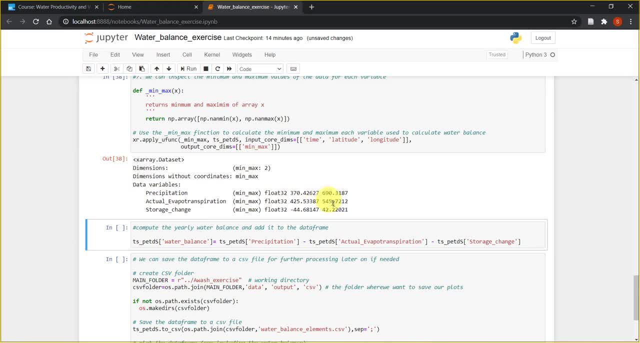 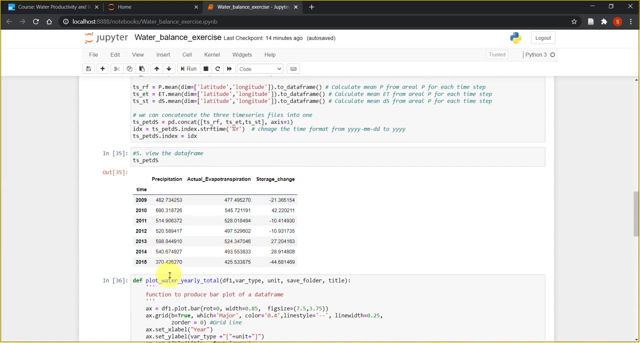 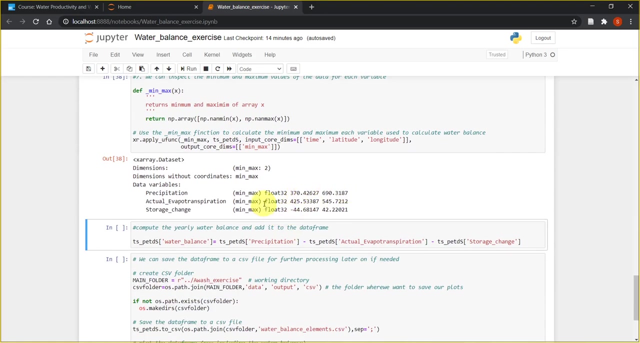 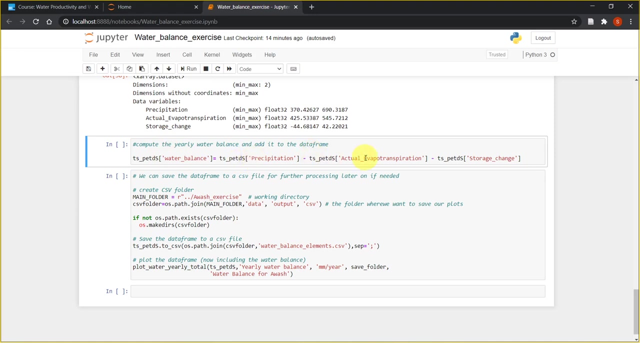 series using this function, so we get like the minimum and the maximum or each input. actually we can visually observe those values from this. but imagine if the time series is very longer, than calculating the minimum and maximum in this way is relatively easy. now let's calculate the water balance. so the water balance we set is equal to the precipitation. 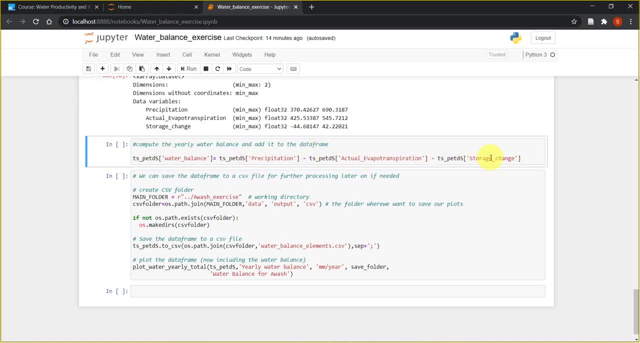 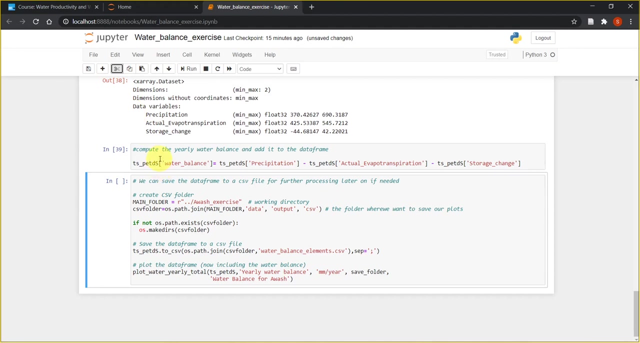 minus the evapotranspiration, minus change in storage. so, if we calculate this, we get the time series, this values for the water balance, and we save it as for the column of the data frame. so we have this. let's calculate and let us look at again how. 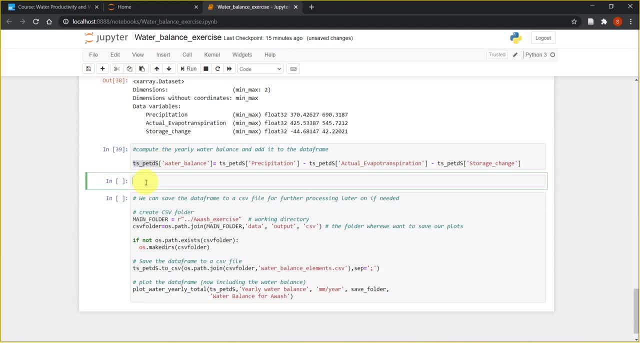 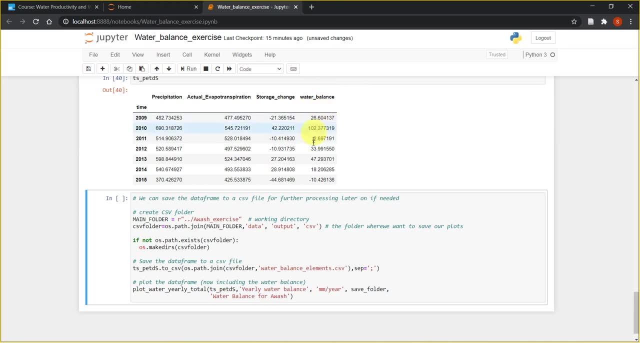 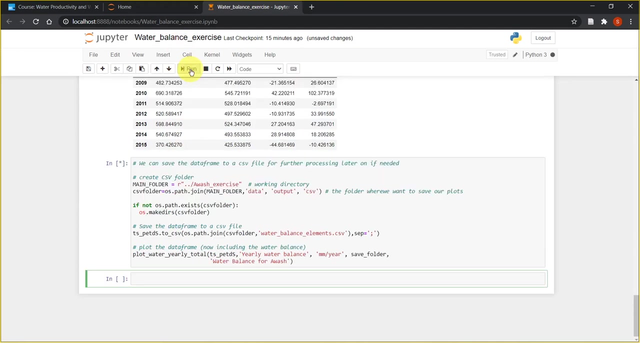 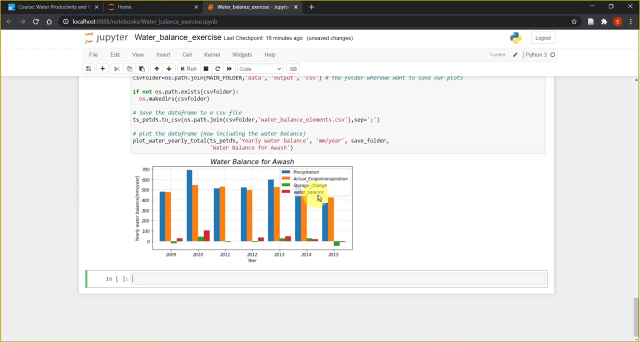 this time series looks like: yeah, you see, now the water balance is added at the first column, so we can also plot this data frame the way we plot it earlier. so let's plot it again and see: yeah, now the plot included the fourth column, which is the water balance. so does the magnitude of the water balance. 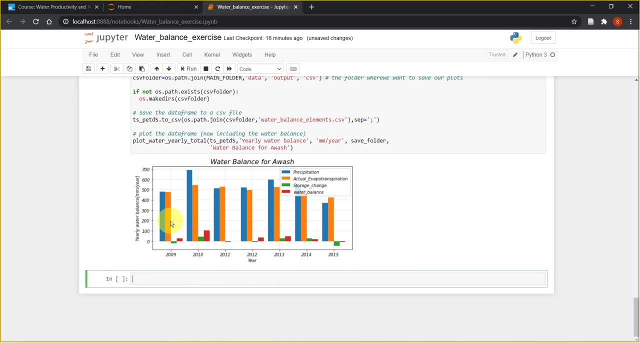 is the same as we expect. no, we expected to have the water balance zero because the basin- we assume the basin is close to the basin and there is no any non-observed outflow, but we have some values of the water balance. so this could be because of two reasons. the first one is because the 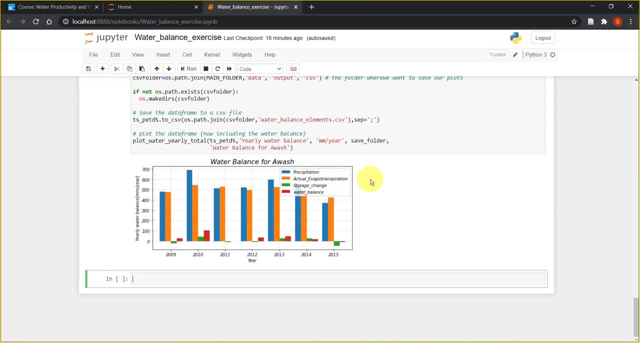 remote sensitive, remotely sensitive estimate of the inputs. the precipitation evapotranspiration in the chain storage involves some uncertainty, so that also can make the water balance calculation uncertain. and the second: the reason could be that even if we say this is a closed basin, there is no known outflow to external. 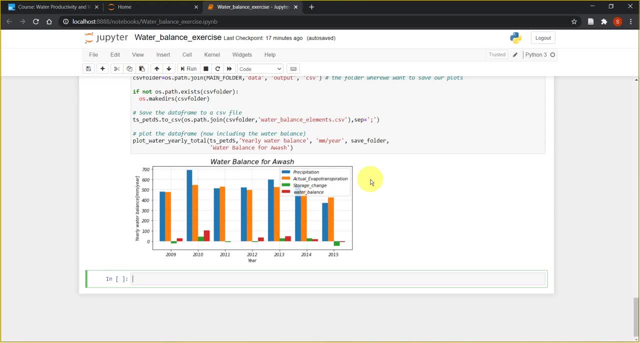 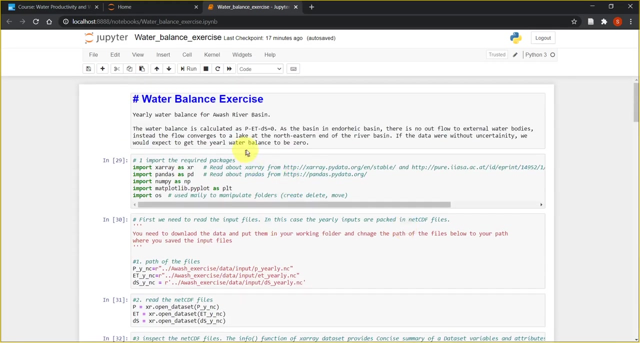 water bodies, there still could be outflow in the form of groundwater from the river basin which we don't have any observation. so because of these two reasons, the water balance could be different from zero. this is how you calculate the water balance of a river basin from remotely sensitive estimates of the inputs. i hope you can manage to run this exercise by yourself.